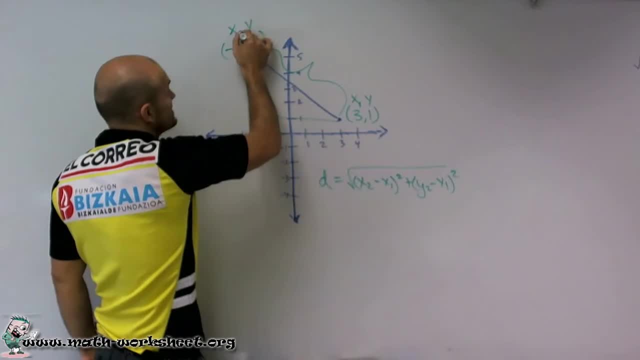 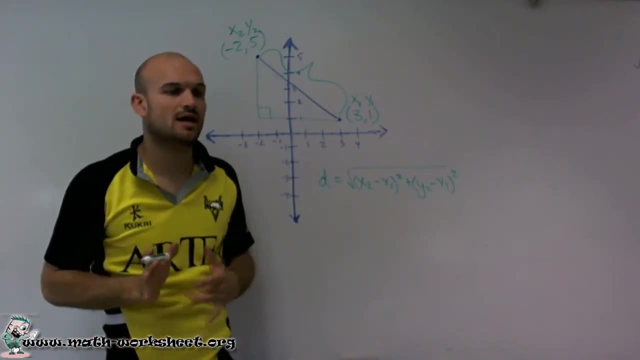 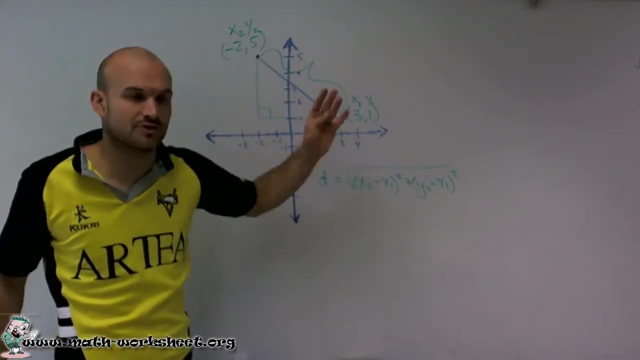 So I'm going to label this x1 and this x2, this y1 and this y2.. It's just a way, using subscripts, to help us differentiate between our variables. So now what I'll simply do- and it doesn't matter which one you pick as 1 and 2,. 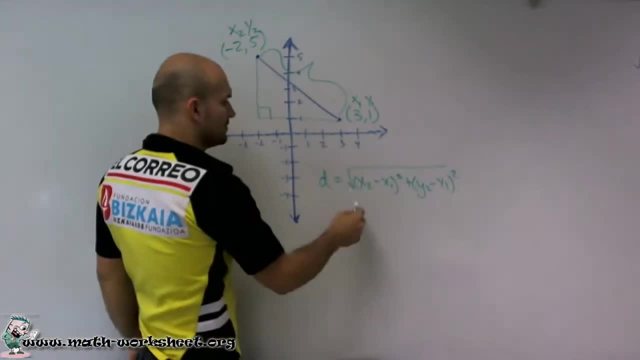 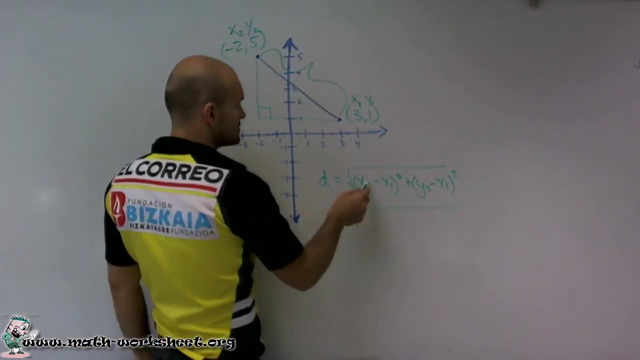 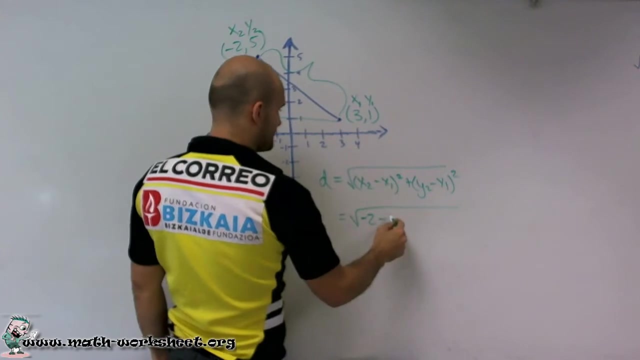 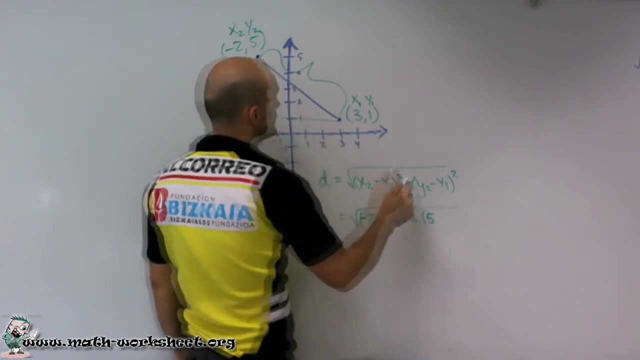 as long as they're the same, you're okay. So now what I'm going to do is I'm just going to plug in my values into my formula. So plus 2,, I said, was negative, 2, minus x1,, which is 3, square that plus y2, which is 5, and minus y1, which is 1.. 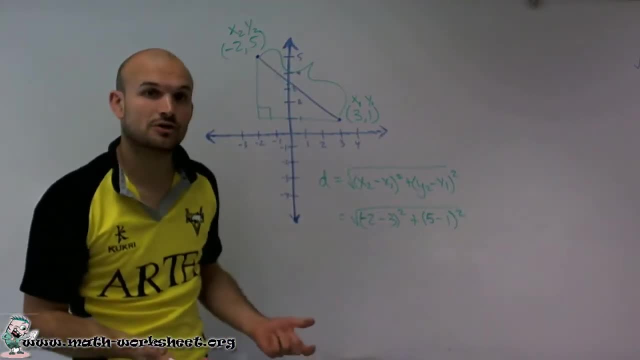 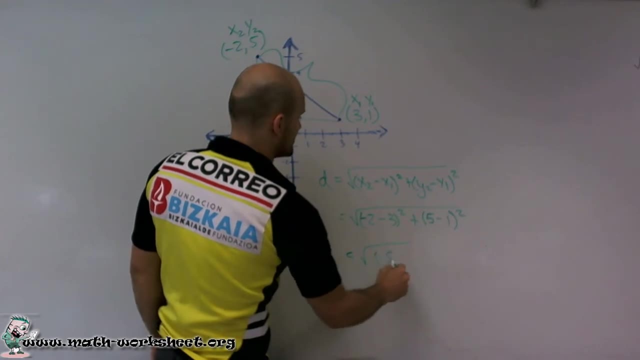 Square it Okay. so now I just need to do a little simplifying. So I have negative 2 minus 3, which is negative 5.. And I know I'm just going to do this a little bit older Just to make sure we all have it. 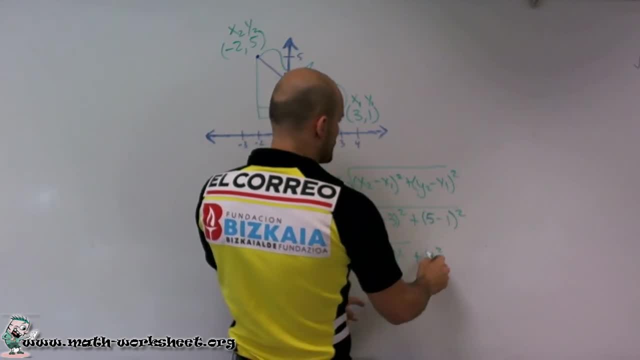 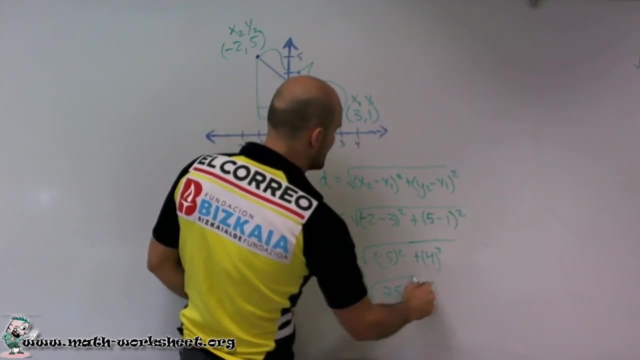 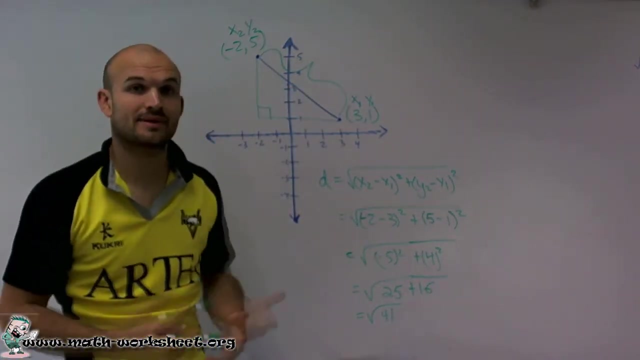 Negative: 5 squared plus 5 minus 1 is 4 squared. So therefore I have square root of 25 plus 16, which equals the square root of 41.. So now I need to determine. you know what is the square root of 41.. 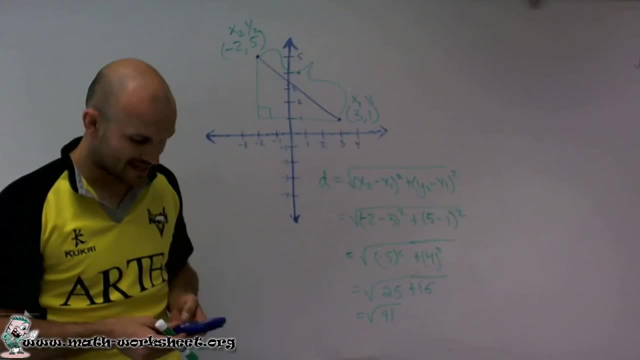 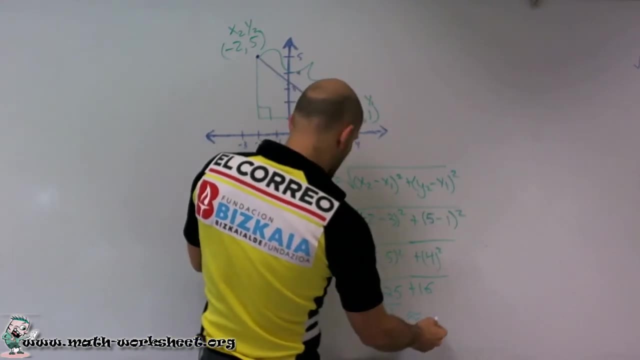 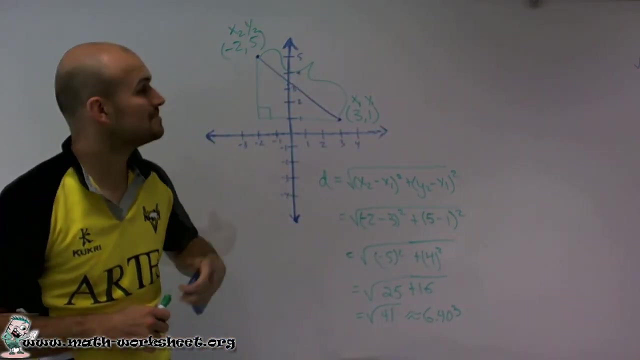 Well, I'm just going to use my handy calculator, because I know that 41 is not a squared number. So the square root of 41 is going to give me irrational decimal And we'll just approximate it to 6.403.. And that is how you find the distance between two points. Thanks. 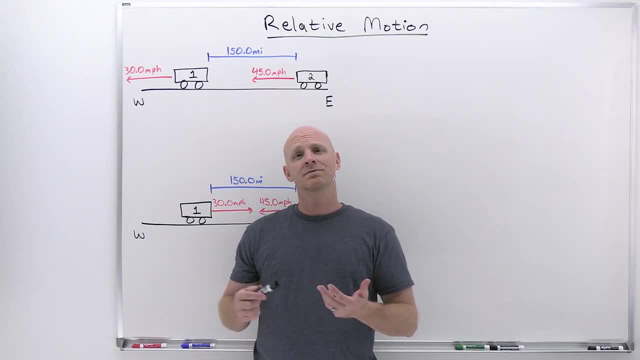 Relative motion is going to be the topic of this lesson. We're going to start with some classical one-dimensional problems involving trains and then we'll move on to some classical two-dimensional problems and we'll see that, just like we've done throughout the rest of this chapter on motion, in. 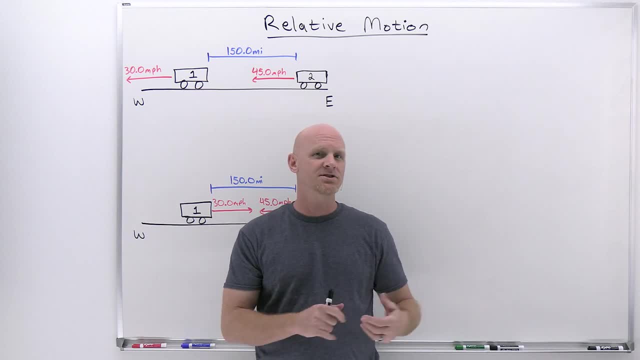 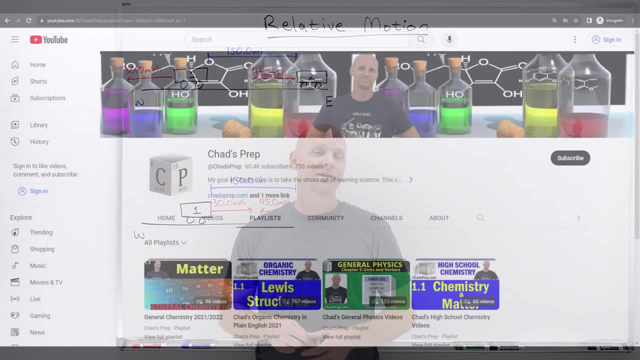 two dimensions. we'll be able to treat the x-dimension and the y-dimension independently. My name is Chad, and welcome to Chad's Prep, where my goal is to take the stress out of learning science. Now, if you're new to the channel, we've got comprehensive playlists for general chemistry.